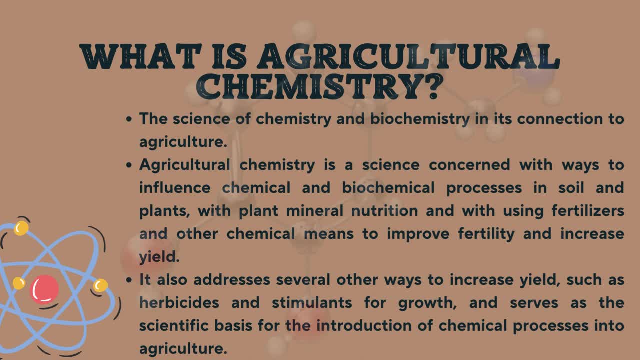 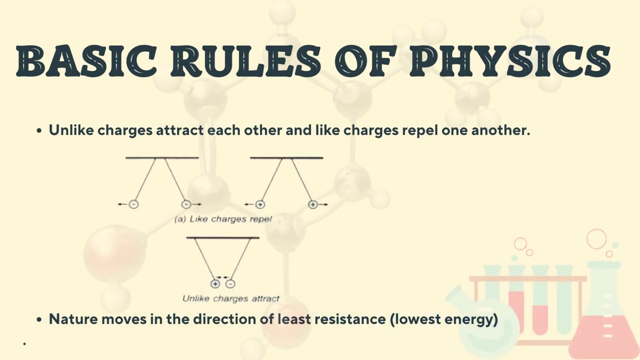 from food production to manufacturing of products like fertilizers. basically, It also addresses several ways to increase yields, such as herbicides And stimulants for growth, and serves as a scientific basis for the introduction of chemical processes into agriculture. This lesson will mostly focus on chemical bonding, as well as inorganic and organic compounds. 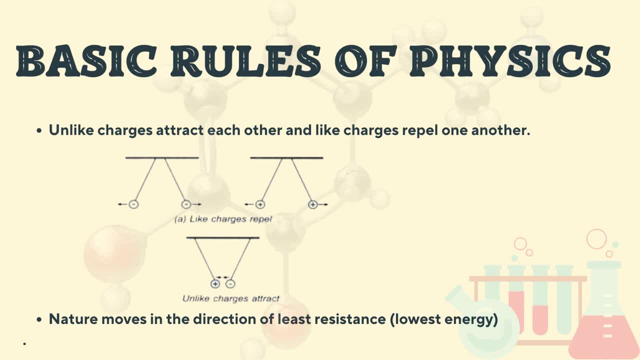 So if you want to understand the basics on atoms, elements, compounds and mixtures, please feel free to scroll down on this channel and find the link in the description. This is the first lesson that I ever uploaded, but I will also put the link down below. 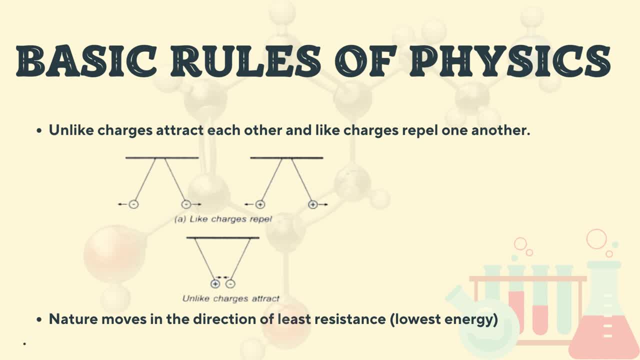 But before we get to the main topics, I want us to understand two basic rules in physics Now. the first one is: unlike, charges attract each other, and like charges repel one another. The second one: nature moves in the direction of the flow of energy. 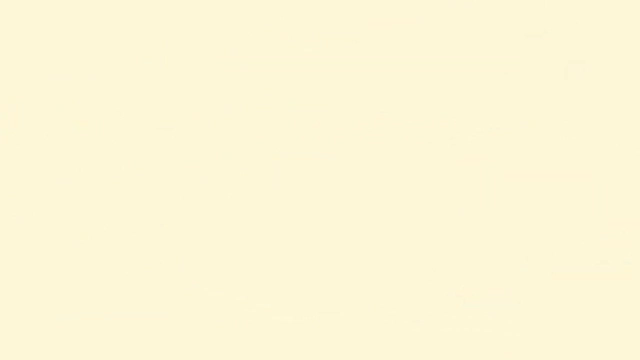 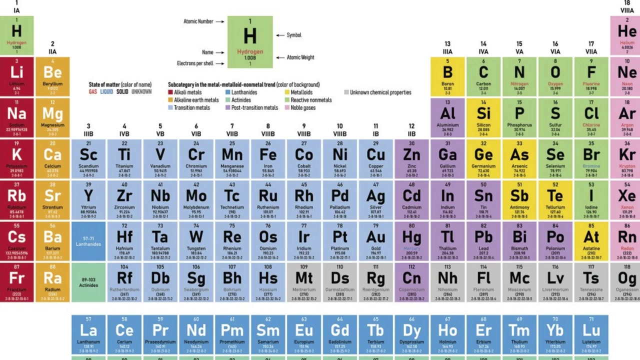 The second one. nature moves in the direction of the flow of energy. The first is the direction of the least resistance. Right Now, I hope you have your periodic table next to you, my darling, because, child, we're going to need it. 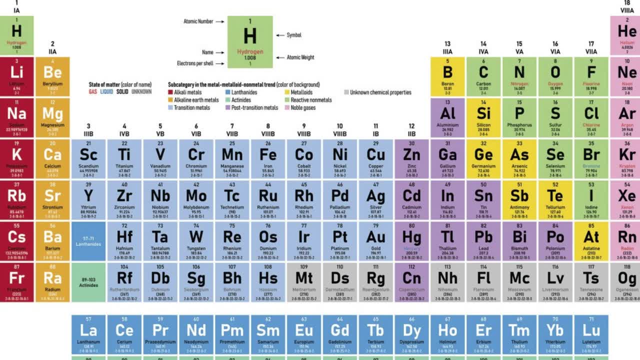 We're going to use it in this session And basically, when you are talking about chemistry, if you have a lesson in chemistry, make sure your periodic table is always next to you, unless you know it by heart. If you don't know it by heart, 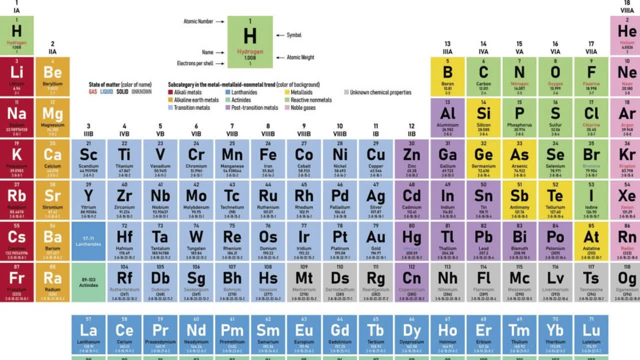 then make sure it's always next to you. I know teachers always encourage learners to know at least the first 20, especially if you are in the senior phase. right, Senior phase, at least the first 20,. but FET phase, FET phase. 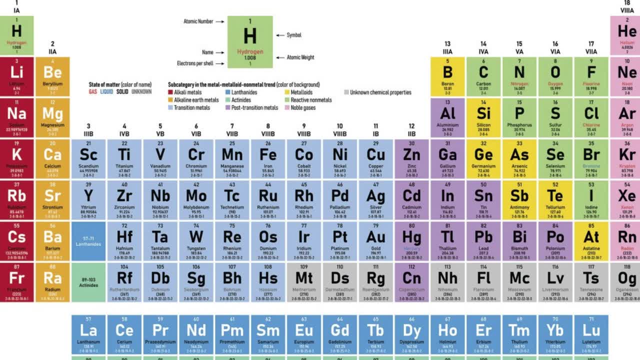 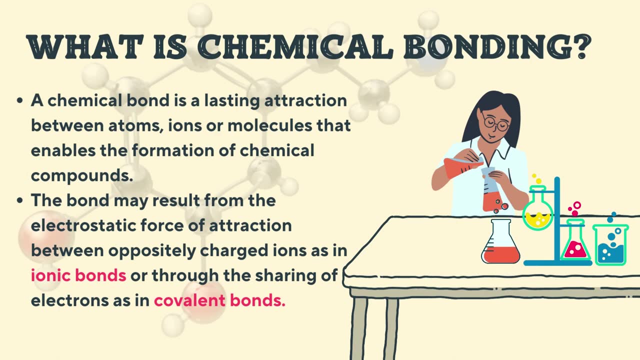 child. I'm not sure if you can be able to know all of them, but it's possible. hey, It's possible to know all of them, but it's also advisable to have your periodic table next to you. So yes, let's get to it. What is chemical bonding? This is basically a process by which 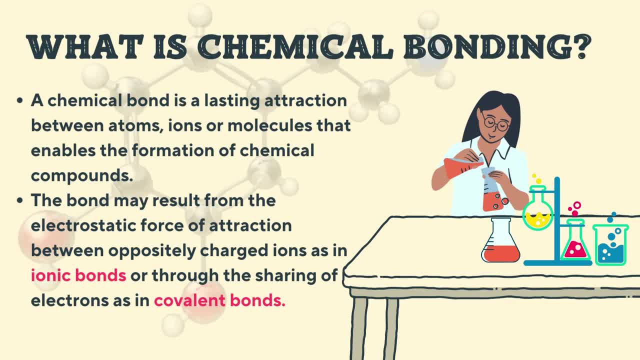 elements combine to form a compound. So chemical bonding is basically the lasting attraction between atoms, ions or molecules that enable the formation of chemical compounds. That is a complex definition, but it's a process by which elements combine to form a compound. 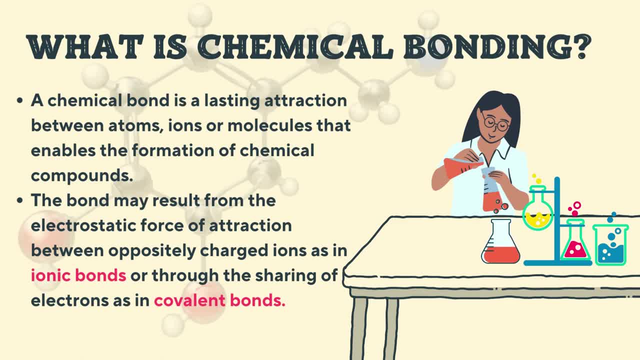 That's the simplest one. you can just say It's a process by which elements combine to form a compound. Then what does this mean? Basically, two hydrogen atoms will combine with an oxygen atom. then they form a water molecule. right, That is a compound. okay, Now the bond may result. 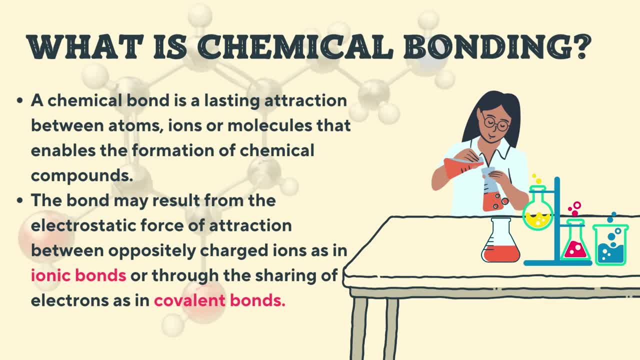 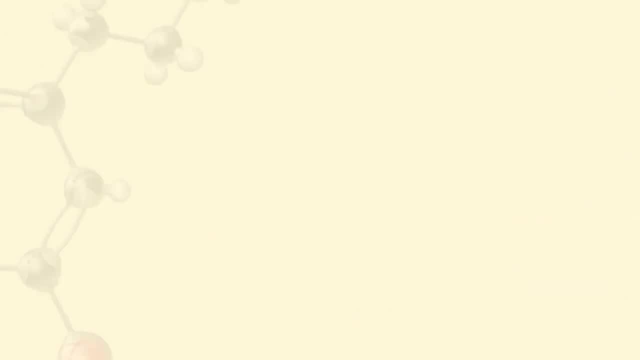 from the electrostatic force between oppositely charged ions, as an ionic bonds, or through the sharing of electrons, as in covalent bonds. Now let's look into this. I just talked about ionic bonds and covalent bonds, So 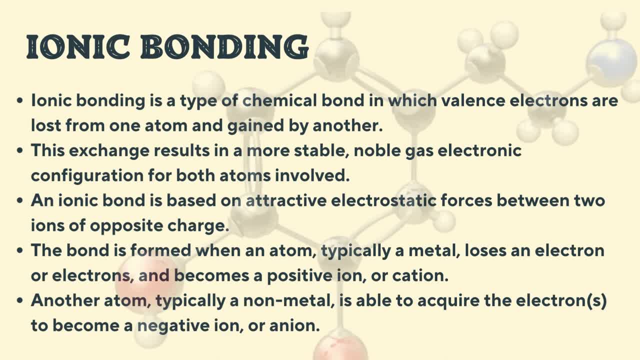 let's start with the ionic bonds. So these are the main types of bonding. We'll just look at them. There are also the other ones, like your hydrogen bonds and other bonds, but for this lesson just focus on two. Now, if we're talking about ionic bonding, right, these are bonds between. 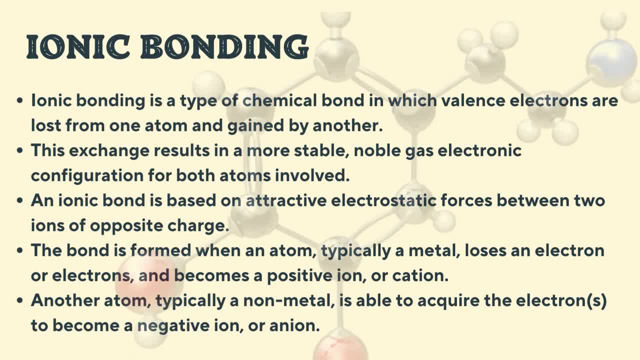 an Athena metal and a metal right. So ionic bonding is a type of chemical bond in which valence electrons are lost from one atom and are gained by another atom. Now this exchange results in a more stable, noble gas electronic configuration for bonding. So these are the main types of bondYes. 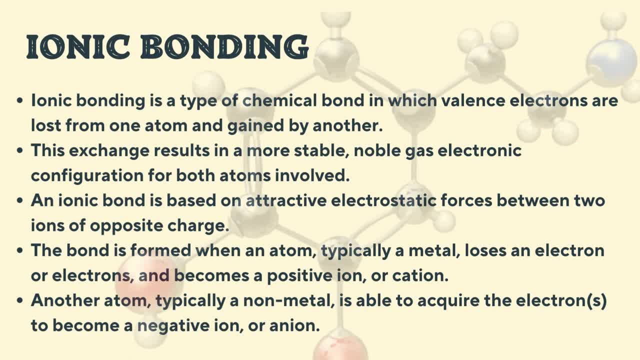 atoms involved. right now, an ionic bond is based on attractive electrostatic forces between two ions of opposite charge. right now, this will include the ket ions and the n ions. now you may ask: what is that now, when a bond is formed? a bond is formed when an atom, typically a metal, 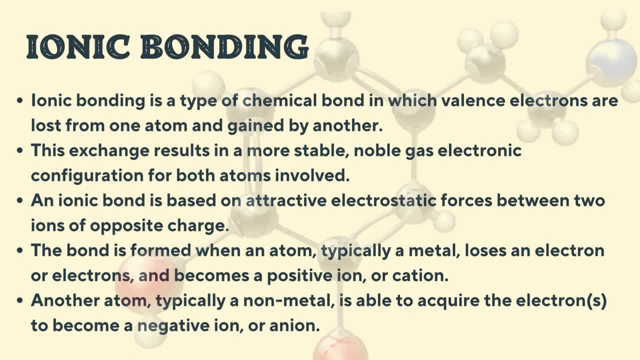 loses an electron or electrons and it becomes a positive ion. right, then we call that a ket ion. so now, when a non-metal now is able to receive or to acquire electrons, it becomes negative, it becomes a negative ion and we call this an n ion. right, so be able to note the differences. 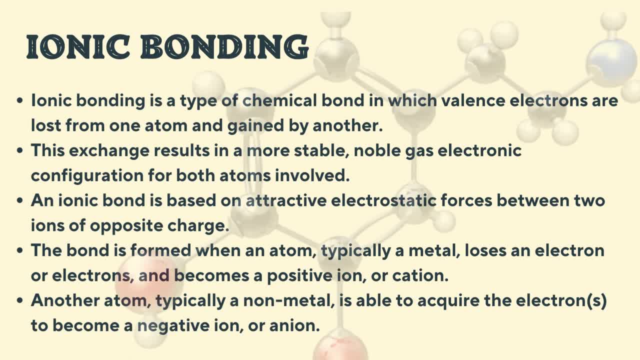 be able to understand the differences. we are talking about an electron that loses a atom. an atom that loses electrons, then it will become negatively charged, it will become a pos, it will become a positive charge- excuse me for that. then we call it a cat iron. but now, if an atom receives electrons, 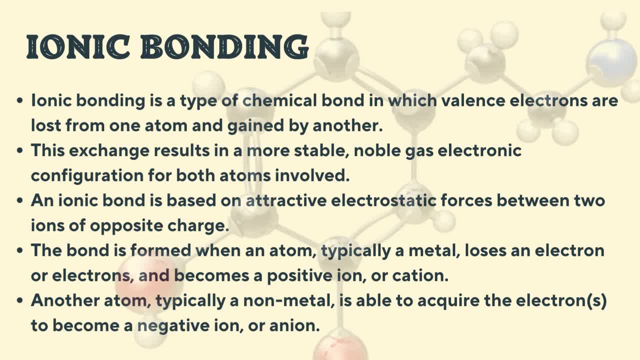 then it will become negatively charged. then we call it an n ion. so remember, the electrons are negatively charged. so when you gain, when they gain more electrons now they become more negative, then there will be an n iron. but when they lose electrons they will become more positive. then they will be called a cat iron. i hope that makes sense. 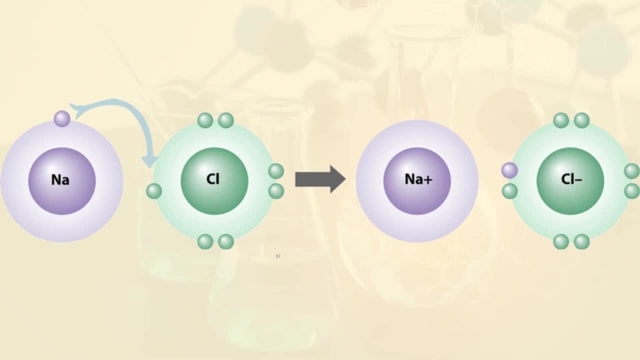 now let's look at the example now of ionic bonding. we're gonna look at sodium here and chlorine right. so what you will notice here is that sodium wants to lose an electron right and chlorine wants to gain an electron. and why is that so? under our shell right, the valence shell, chlorine has got seven electrons. 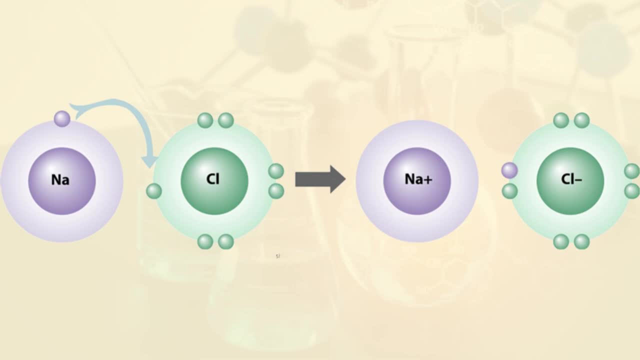 and it's supposed to be eight, right. and then now it needs one electron. so what will happen? sodium is willing to give up its electron to be transferred to chlorine. so these trading now, right now, as soon as sodium transfers this electron, sodium will become positively charged. then what will happen now to chlorine? 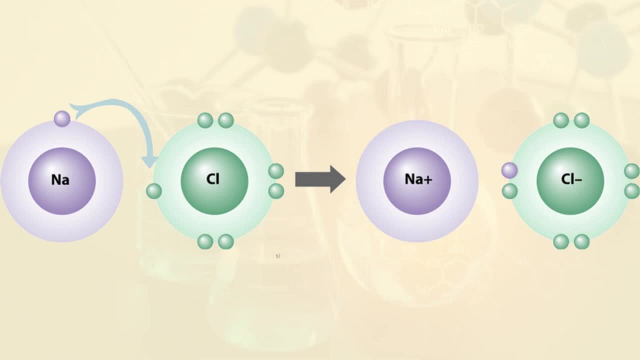 because chlorine has received one electron from sodium, then it will become negatively charged. then the two of them, now they will be attracted to each other because the other one is positive, then the other one will be negative. then there will be this force now that is attracting them to. 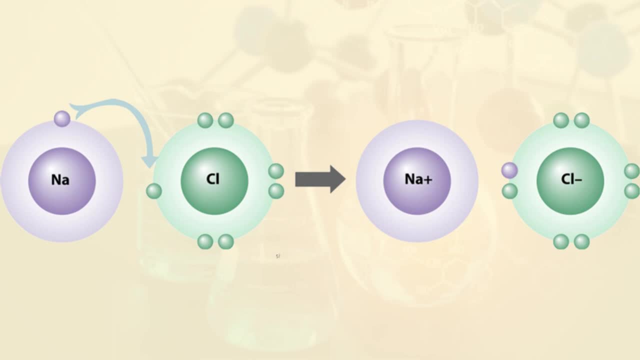 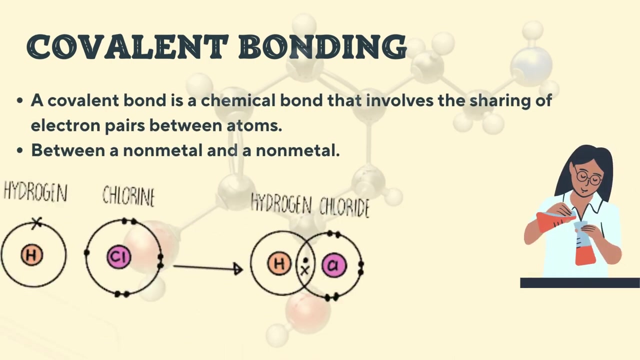 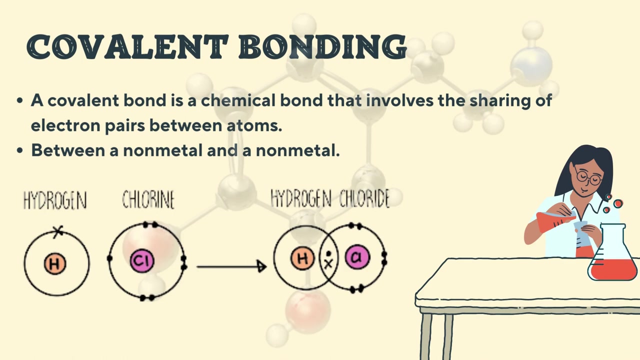 one another. remember i said one of the basic rules is that, unlike, charges attract each other and like charges repel each other. right then, let's get to the second type of bonding, which is coverland bonding. right now, this is the type of bonding that involves now the sharing of electrons. so, in the chemical bonding, as i have, 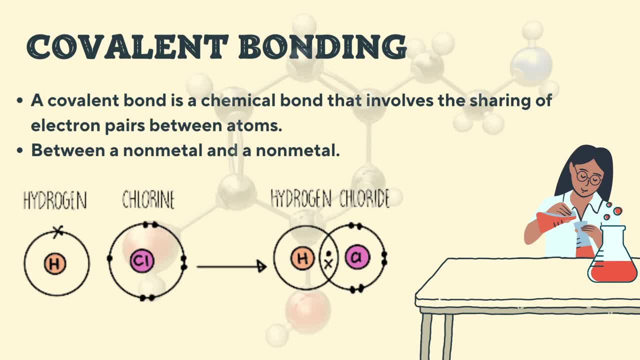 mentioned earlier, there is sharing of electrons and there is transfer of electrons. so, unlike ionic bonding, where there was trading or transfer of electrons, here we are sharing. right now these atoms are sharing electrons. so this bond occurs between a non-metal and a non-metal, right non-metal and another non-metal right now when we're talking about, if you look at the 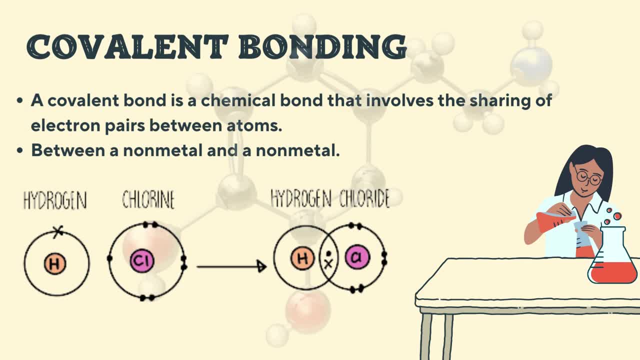 the example below: the hydrogen and chlorine uh bonding. what is happening here? we have a hydrogen, which is a reactive non-metal, and we have a chlorine, which is also a reactive non-metal, and they both need electrons, or one electrons each, because if you look at chlorine, it has got seven electrons on the valence shelf right, so they will now be sharing. 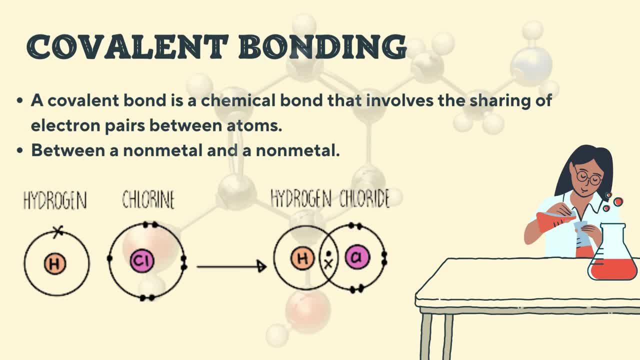 this electron or these electrons so, and that will give hydrogen its steward, and that will give chlorine its octet. now, with the octet rule, with the jewish rule, that's that day- it states that the hydrogen and helium may have no more than two electrons in their 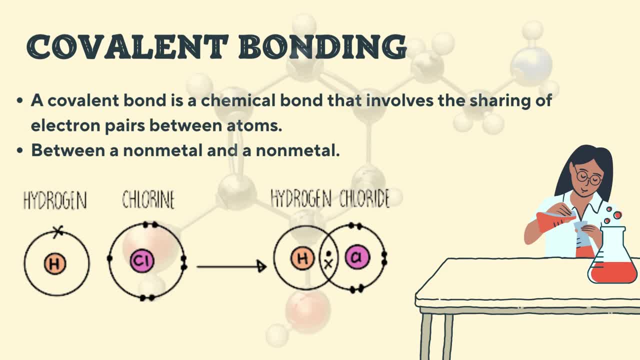 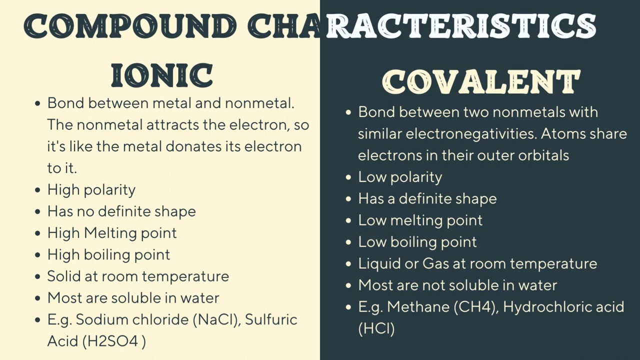 valence shelf. but now remember, we said um, chlorine will have its octet, now with the octet rules. basically, it refers to the tendency of atoms to prefer to have eight electrons in the valence shell. i think i have mentioned this earlier then let's move now to the characteristics of 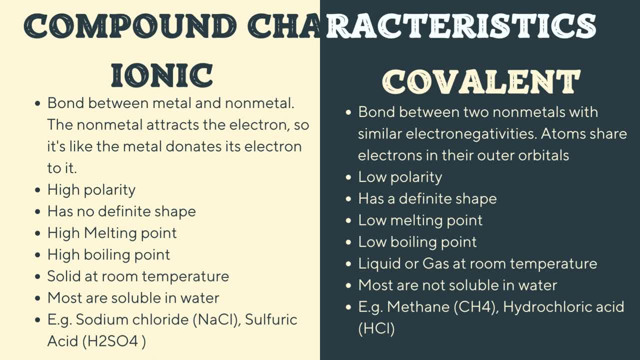 these two um bonds, or the compounds that are formed by these two bonds, right, both ionic bonds and covalent bonds. so if we're looking at ionic bonds, as we have mentioned earlier, this is a bond that occurs between a metal and a non-metal. but with covalent bond, it occurs between two non-metals- right, so they will be. 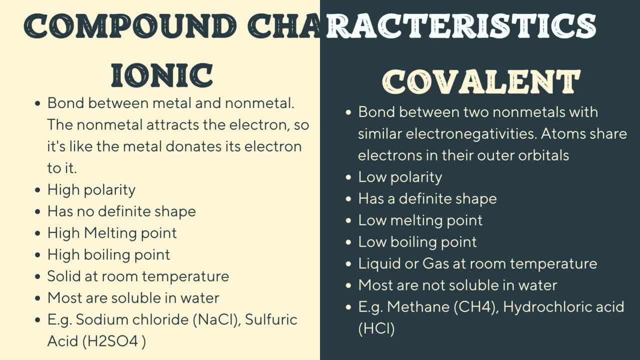 sharing of electrons here on their outer orbit orbitals, but with ionic bonds, one will donate to the other. then, if we're looking at the polarity, if we're looking at melting point as well as boiling point, ionic bonds or compounds that have ionic bonds- 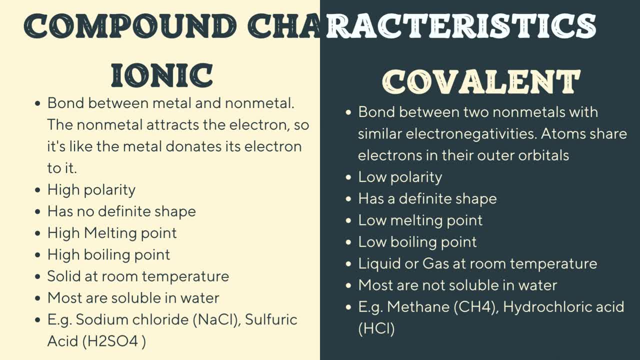 will have high polarity, high melting point and high boiling point. but with covalent bonds they will have low polarity, low melting point and low boiling point. and when it comes to shape, now compounds that have ionic bonds will have no definite shape, but compounds with covalent bones. 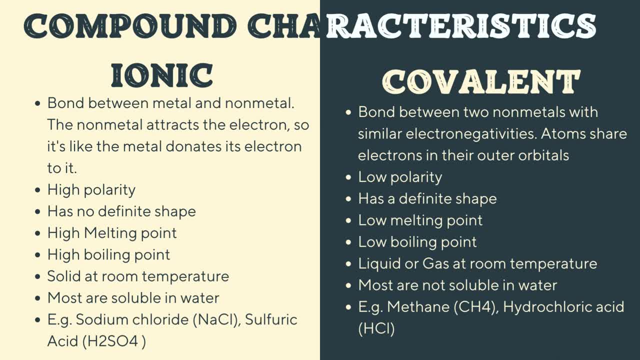 in them they will have a definite shape and they will exist either as a liquid or as a gas at room temperature. but with ionic they will exist as solids, as at room temperature, and they are more soluble in water. but compounds with covalent bonds, most of them, are not soluble in water and the examples are methane, the hydrochloric acid, 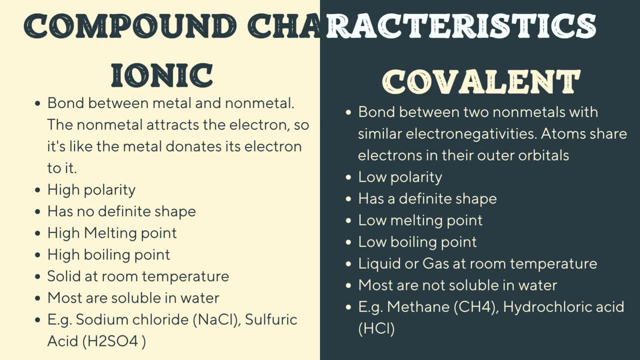 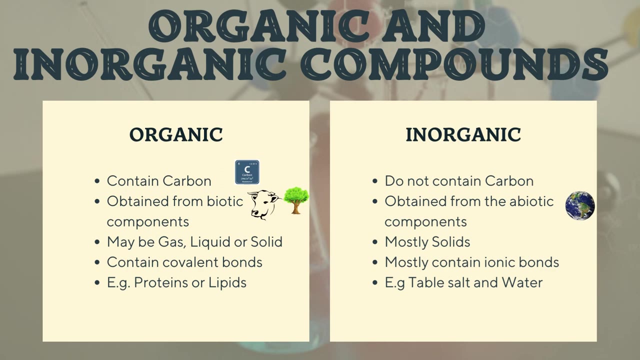 but with with ionic bonds. examples: um include one we have um mentioned earlier, the sodium chloride, as well as sulfuric acid. but those are not the only ones. they're not limited to these ones. i have to just select two, and then let's move now to organic compounds and inorganic compounds. so